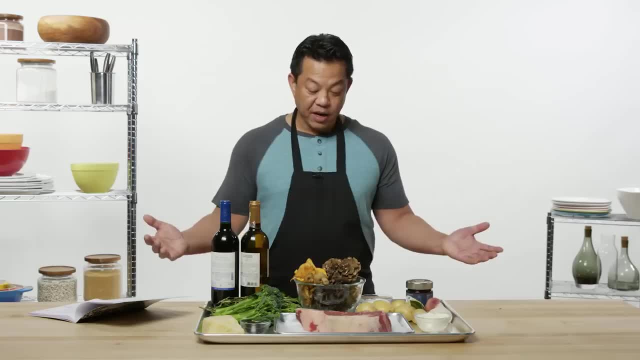 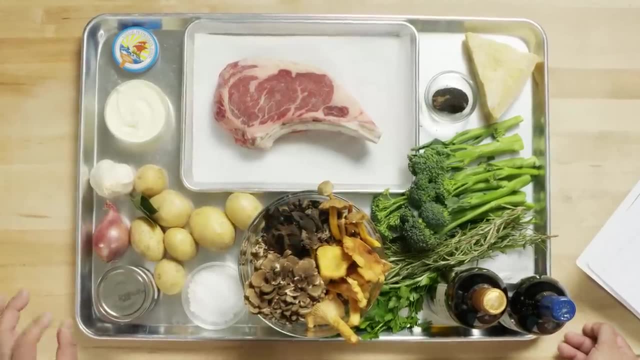 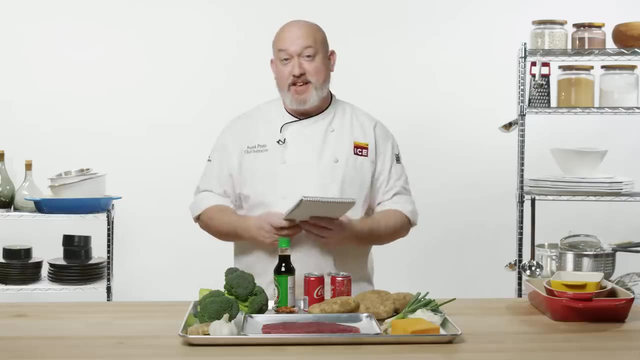 I feel slightly evil. It's like we broke into a five-star Michelin restaurant and I just grabbed everything I possibly could and said: let's have some fun With Lorenzo's recipe. I have a little more simpler ingredients and maybe something that's a little more commonplace. 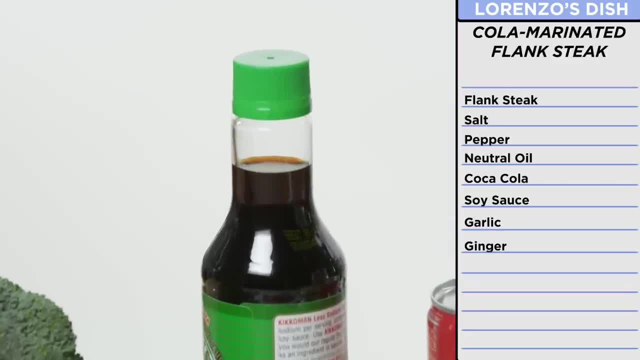 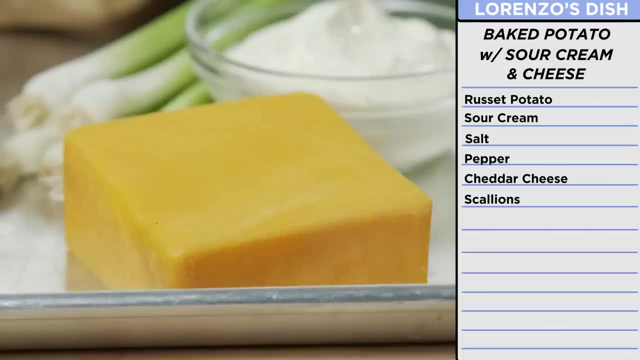 in your kitchen: Flank steak, Coca-Cola, low-sodium soy sauce, garlic, ginger, broccoli, some chili flake, russet potatoes scallions, sour cream and cheddar. So these ingredients might be a little simpler. 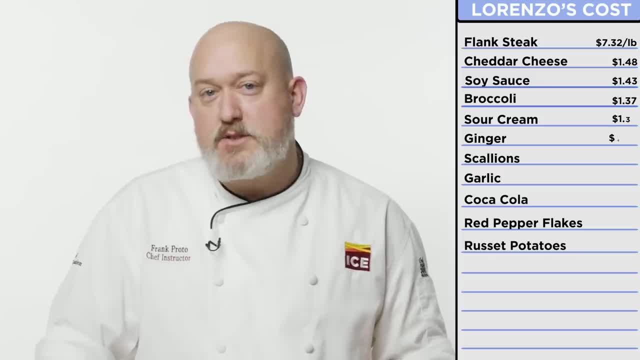 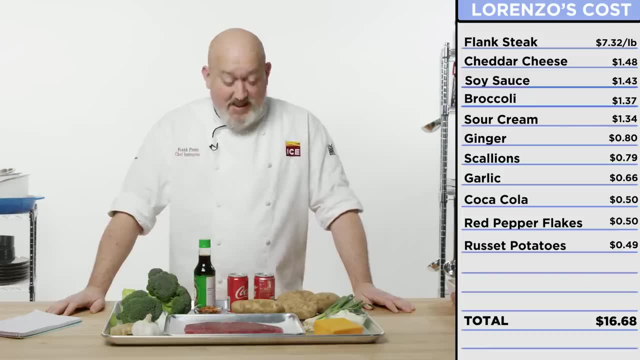 but I think that I can elevate them and make them a little better. If I had to guess, this would probably cost about 25 to $30.. Oh, 16, really. Oh, that's cheaper than I thought. It's a little intimidating. 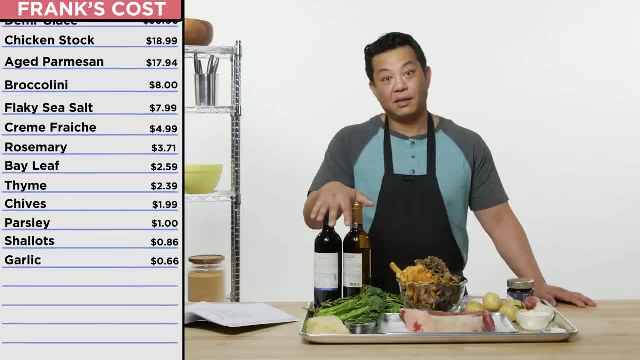 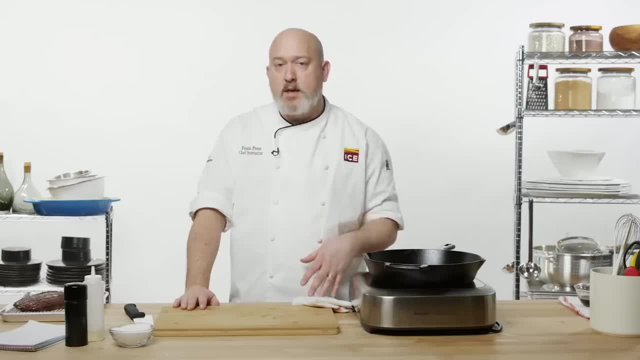 because it's really fancy, schmancy, bechancy. I mean it's a few hundred bucks that I don't have The fondant potatoes. I plan to make sound really fancy and I hope Lorenzo doesn't get scared off by that. Why, why? 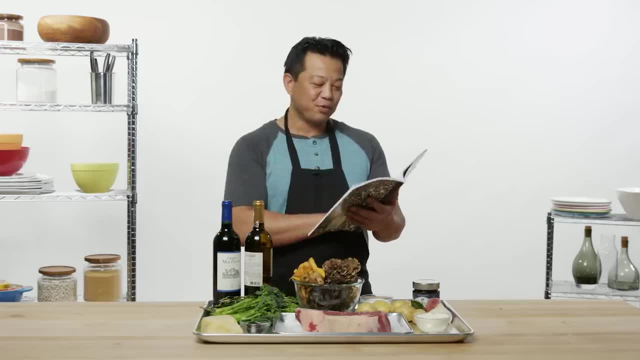 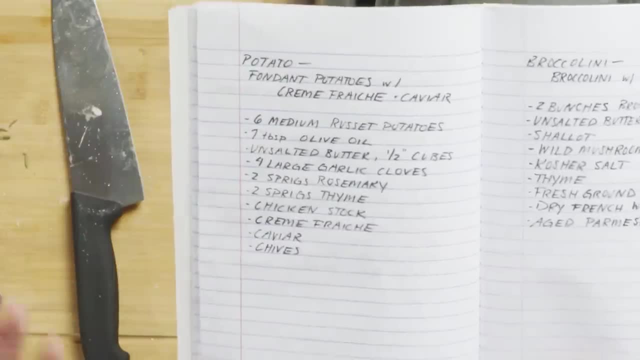 Salt, pepper, butter, potato, simple. What's wrong with you? I like how I'm looking at Frank's recipe. It's actually just ingredients. It doesn't tell me step-by-step stuff. I'm like I think I'm just looking for some help. 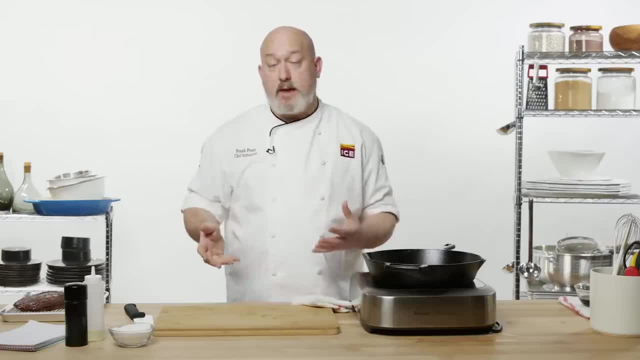 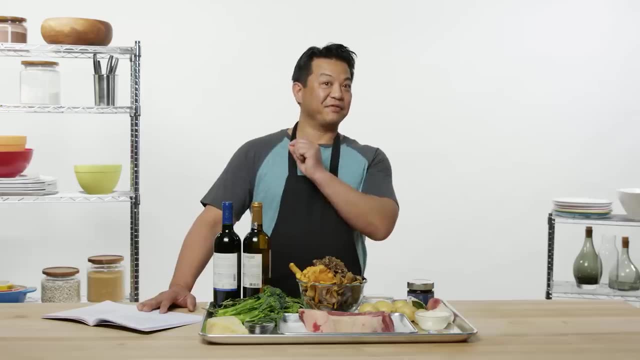 And it's kind of just that next step up from just roasting potatoes in a pan. I'm a little I'm clueless on a couple of things. Is there a chance that I could maybe ask somebody for a little help? Rosemary. 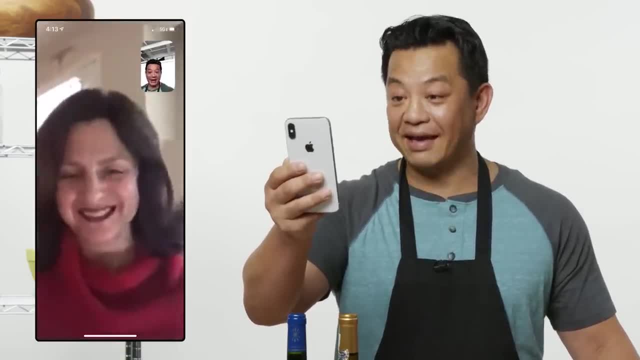 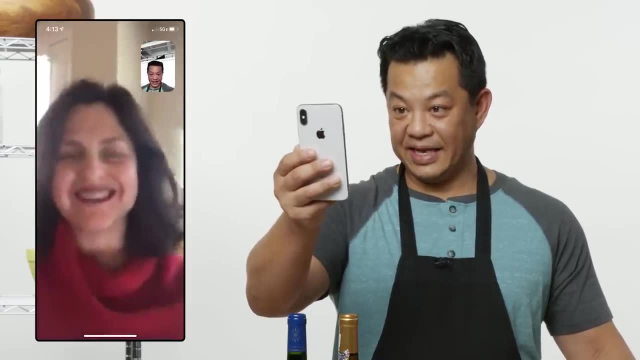 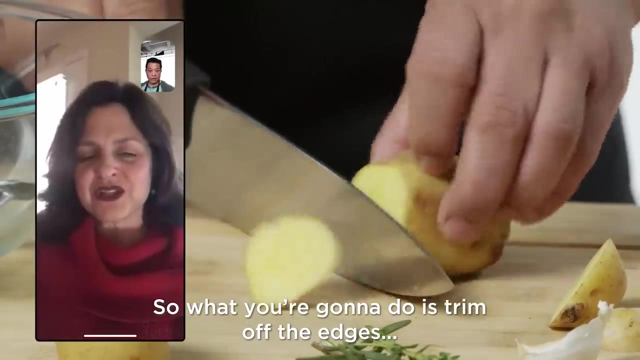 How are you? How am I? I'm panicking a little bit. actually. I feel like I'm on an island and I just drew help in the sand. Can you Fondant potatoes? Oh, they're delicious. What you're gonna do is you're gonna trim off the very edges. 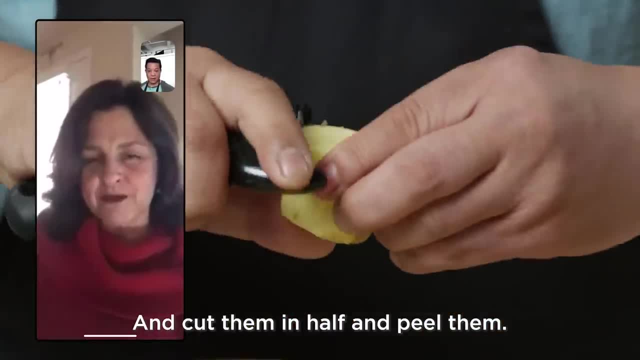 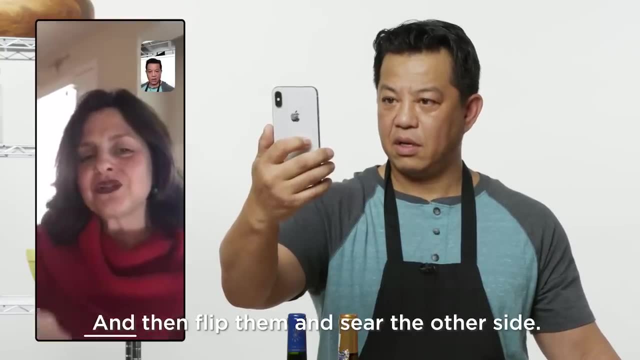 And you're going to cut them in half and peel them- They're gonna look kind of like scallops- And sear the top. get it real crispy, Okay. And then you're going to take them and flip them, sear the other side. 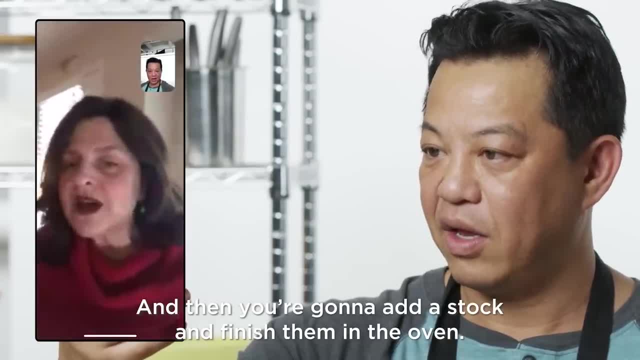 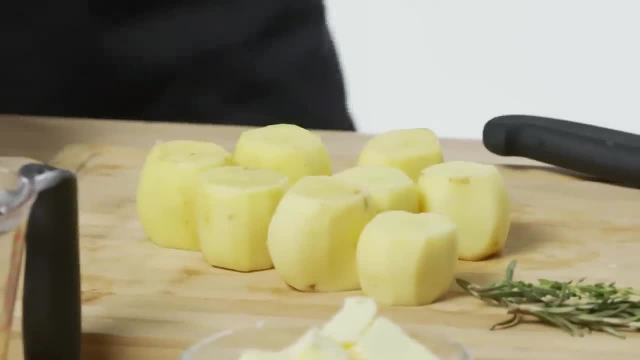 Okay, And then you're gonna add a stock, like a chicken stock or a vegetable stock, Okay, And finish them in the oven. Thank you so much, Rosemary. I appreciate it. Take care, It just sounds more complicated, but it's potatoes. 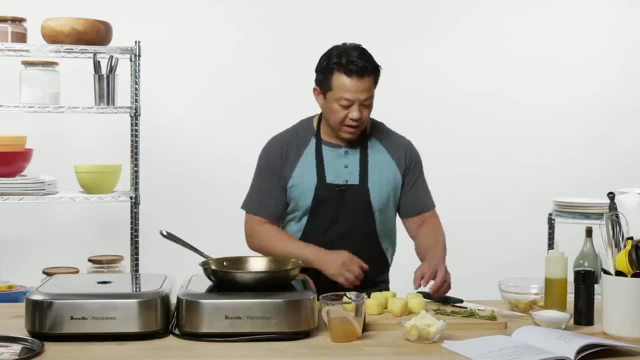 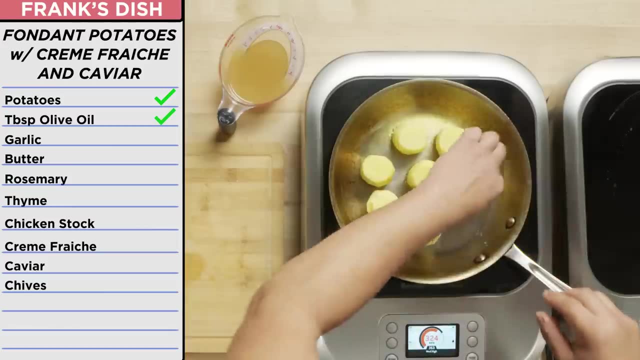 You know I can do it. Bing Ooh, Lord, have mercy. Okay. So I've got all my lovely russet potatoes, pretty much like little stools, And I'm gonna sear both sides. Originally, Lorenzo planned for this. 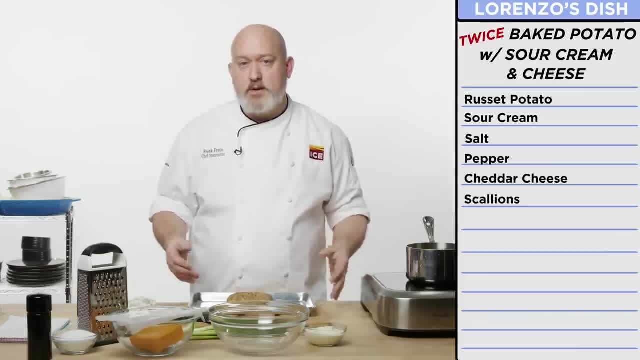 to be a regular baked potato. So what we're gonna do is twice baked potatoes: A little more fat, a little more flavor, just a little more deliciousness. okay, Baked potato butter's great Twice: baked potato with cream cheese and cheddar. 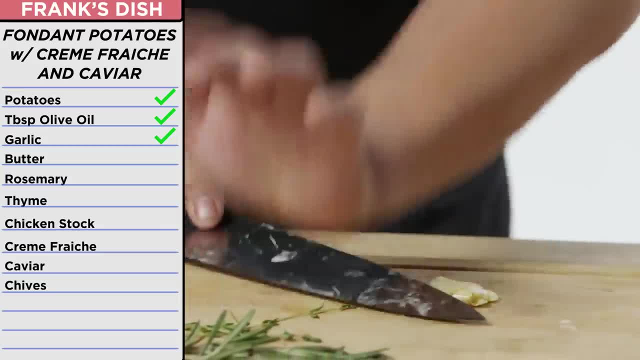 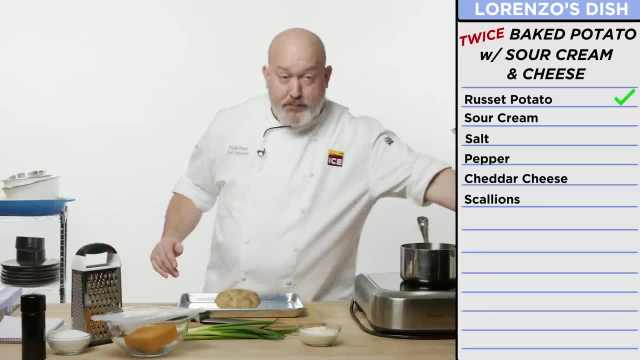 is even better. All right, so I have the garlic, I'm just gonna crush it. I have the ingredients and I know, Just doesn't tell me how to put it together. That's the mystery. First thing I'm gonna do is I'm gonna bake it. 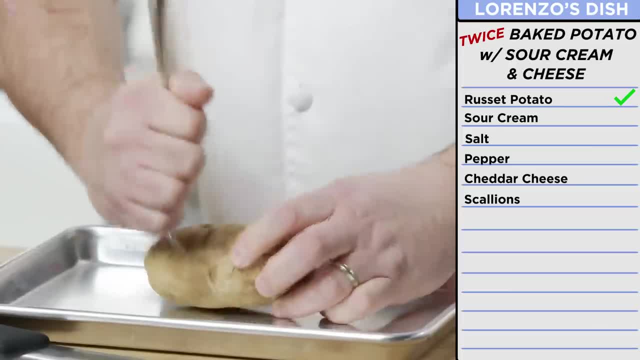 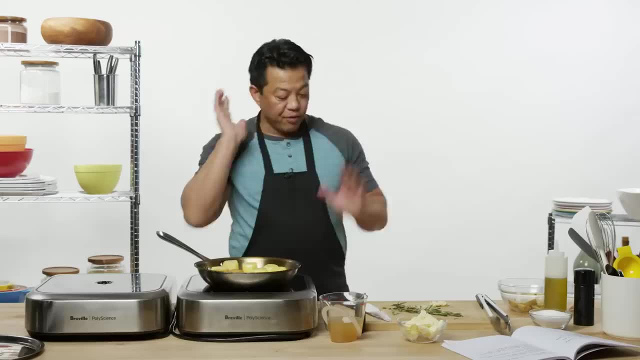 I'm gonna poke a few holes in it just to let steam escape, so my skin doesn't rupture. I'm gonna wrap it in foil. I'm gonna bake this potato about 350, 45 minutes to an hour. I already hear Rosemary saying that's not long enough. 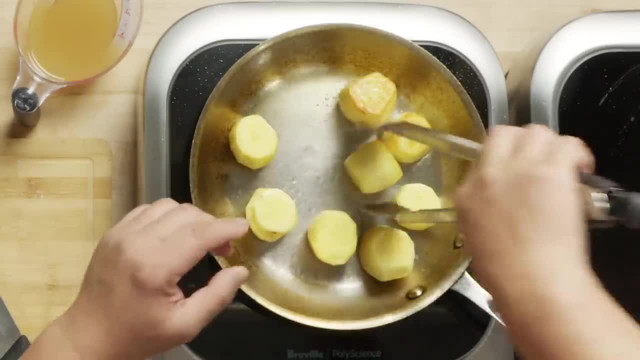 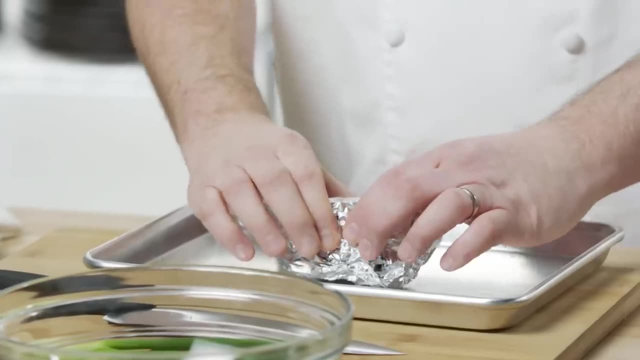 It has to be darker And you didn't sear it long enough. And this is a gigantesaurus tongs- What the heck. So this potato was baked for about 50 minutes. When you squeeze, you can see there's a little bit. 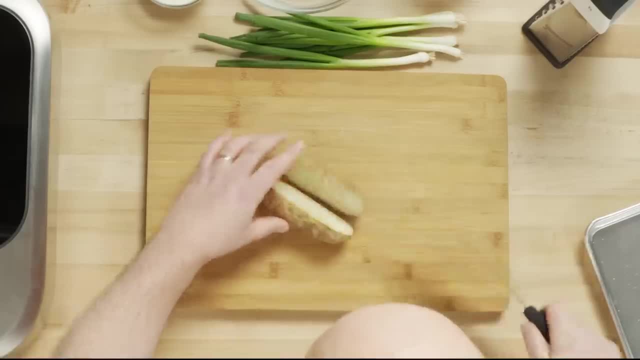 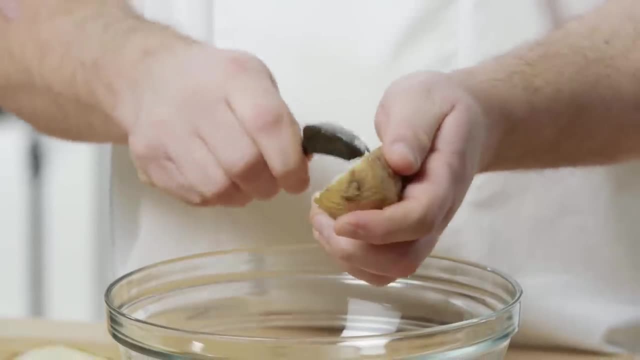 of give. So what we're gonna do is we're gonna take the potato, slice it in half and very carefully- with not trying to break the skin- I'm going to take the center of the potato out. I wanna leave a little bit of a wall there. 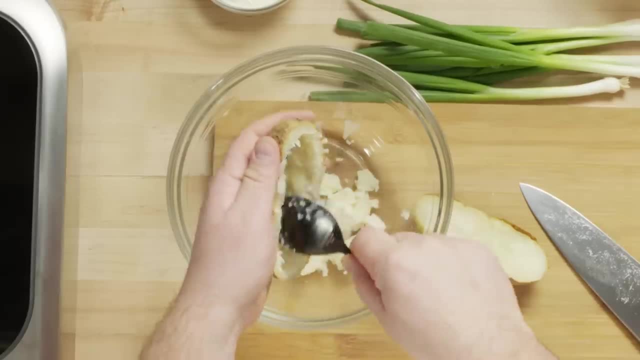 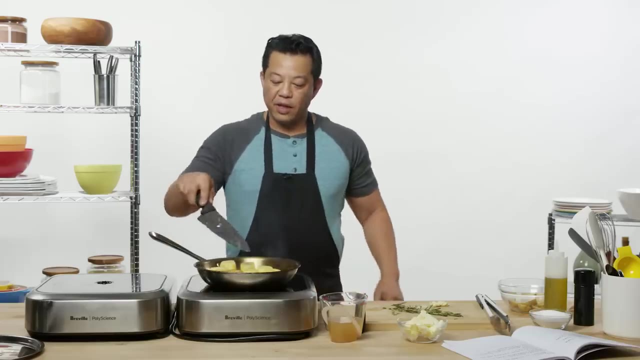 so it's not just skin, just so that it holds together. And I'm just gonna kinda mash this up a little, just so I don't have any big chunks. Yeah, see, I should've turned it up all the way. That's more like it. 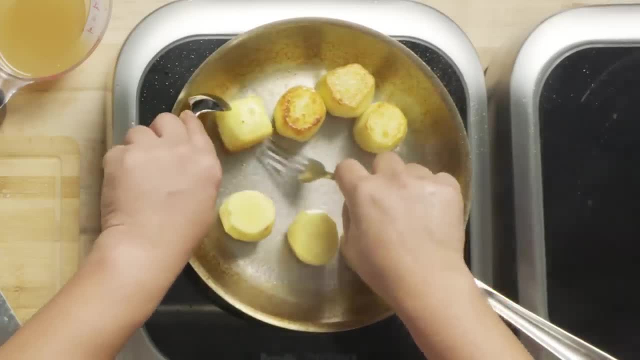 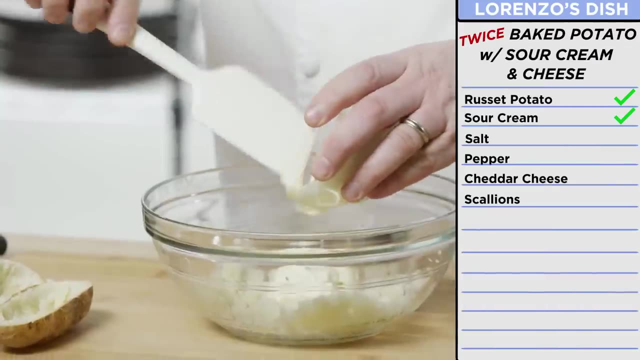 Oh, there you go, hello. That is all right. Rosemary would be happy with that. Okay, okay, okey-dokey-fo-dokey, I'm gonna add all my flavorings to this. A little bit of sour cream. 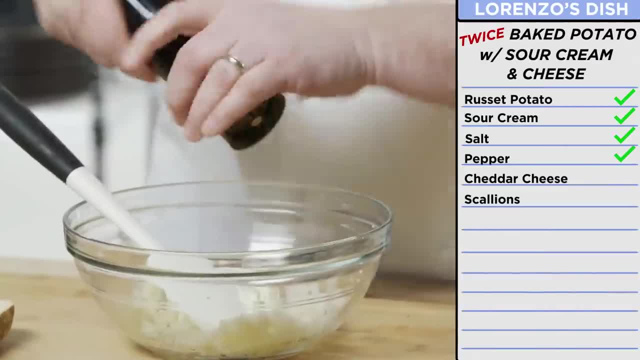 Well, maybe not a little bit, maybe a lot Salt and pepper. definitely We're gonna grate a little cheese. I got some nice cheddar here. Don't be skimpy with the cheese. It's gonna add some richness, a little bit of sharpness to this. 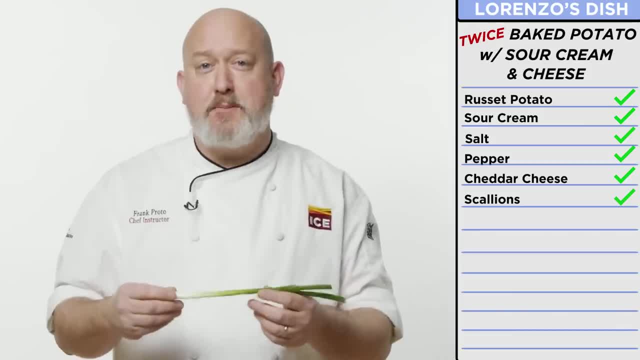 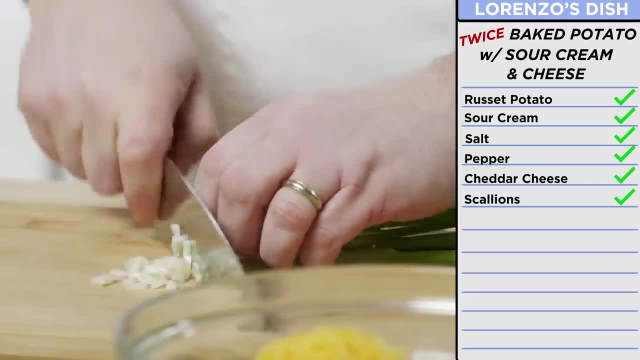 I'm gonna use scallions as a flavoring for this. This is one of those ingredients that people will do this. They'll cut the root end off. They'll either use all the white and throw away the green or use all the green and throw away the white. 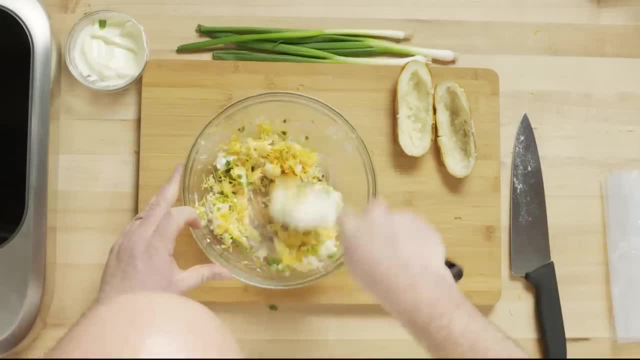 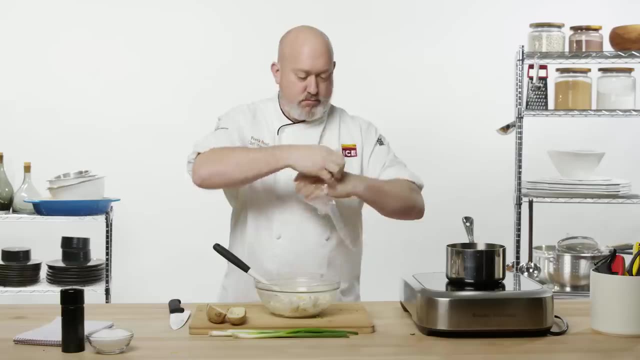 I use the whole thing. All of it's good And we're gonna mix it really well. Always taste your food Delicious. At this point you can probably just scoop it in with a spoon. I'm gonna use a pastry bag, okay. 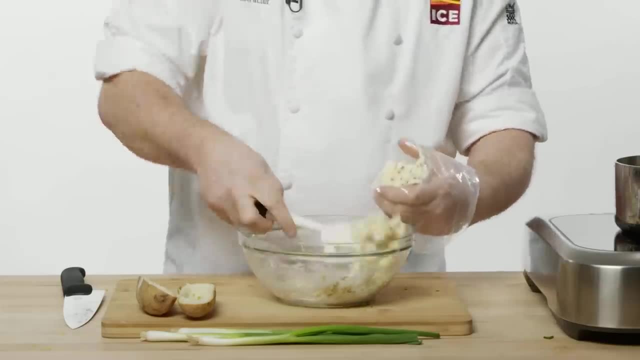 It gives me a little more direction. I can make it exactly the way I want it. It doesn't look like you didn't care and just kind of flopped it on there. The pastry bag gives a little more of a elegant feel to it. 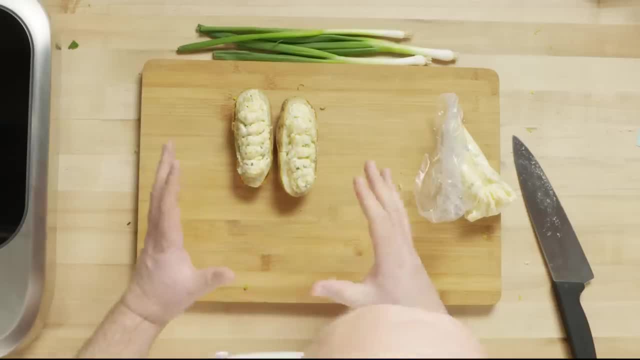 So at this point we're gonna put them in the oven and we're gonna let the top get a little brown, let them warm through and then we'll garnish later. I need to turn this down because I don't want to burn my butter. 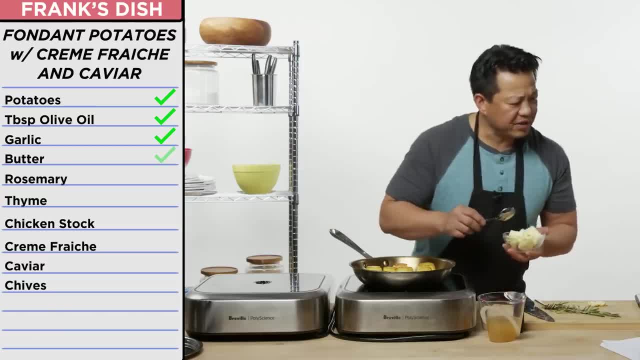 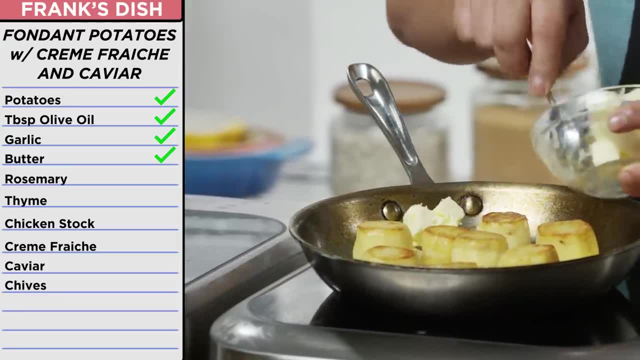 I'm not sure how much butter is in here, but I would imagine- yeah, of course, you add the butter first. I'm guessing that's one tablespoon, two tablespoons, three tablespoons, four. Oh, I'm going for it. 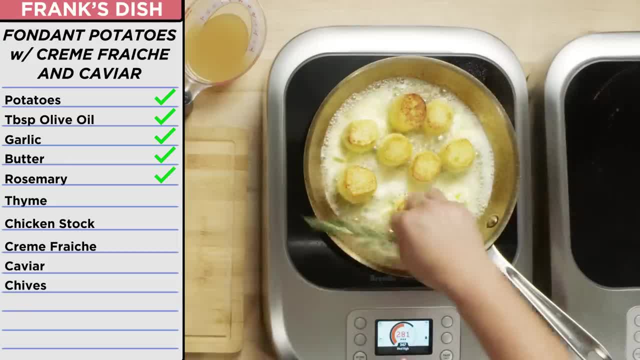 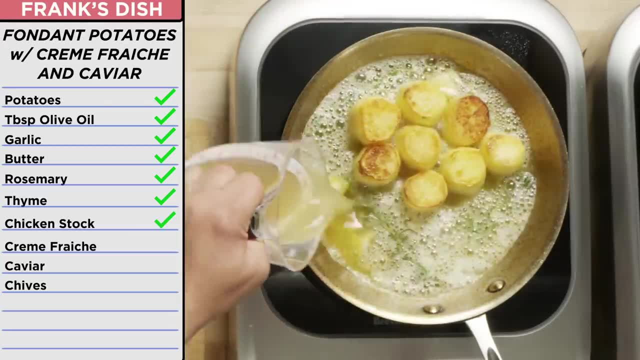 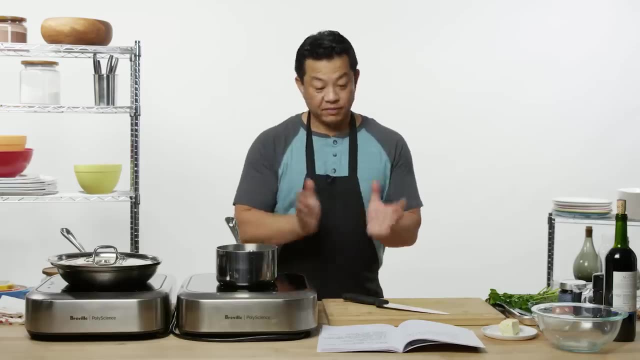 It's like a stick of butter. I think Let's let that go. Oh, let me put my yeah. Oh, that's happening. I mean potatoes and butter. You win Rosemary Pugs. We are moving on to the sauce that I have. 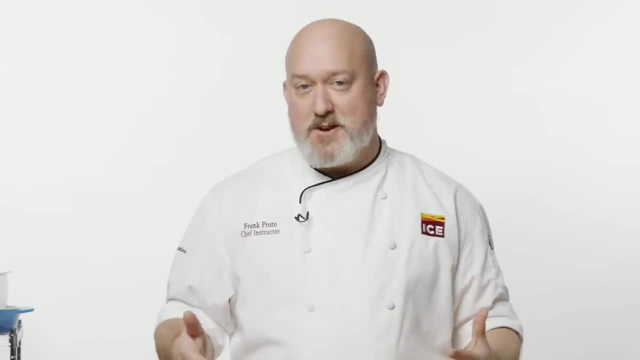 no idea how to pronounce Bordelaise sauce. Thank you, Frank. In Lorenzo's recipe he marinates the steak and the Coke and the soy sauce. I'm not gonna do that. So what I'm gonna do is I'm gonna take the marinade stuff. 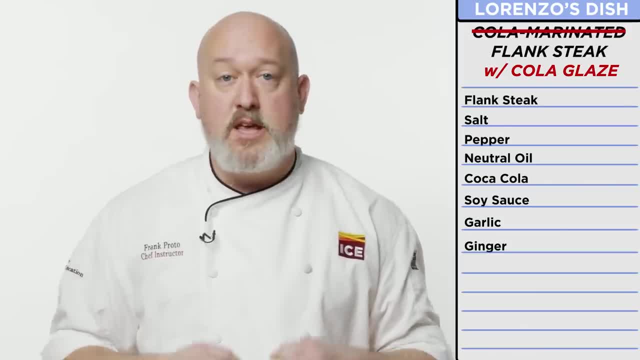 and make a glaze out of it. So if you want to dip into it later, you can dip into it. If you want to just taste a nice piece of meat, taste a nice piece of meat. Hopefully no one shook this up. 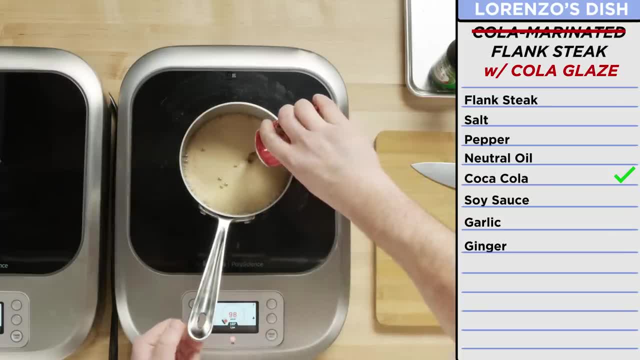 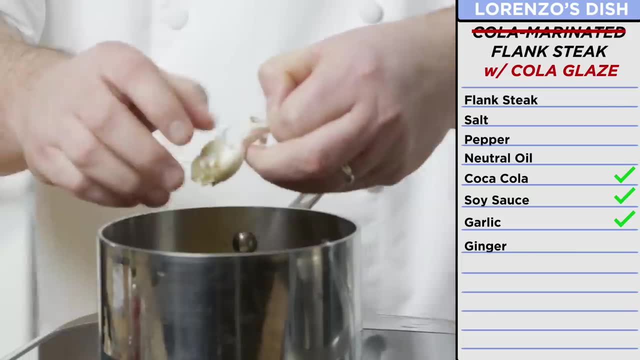 So in places that I've seen Coca-Cola used in marinades and baking, it usually comes from the fact that there was sugar rationing during World War II. So I'm gonna cook this down, basically just dumping everything to the pot and letting it reduce down. 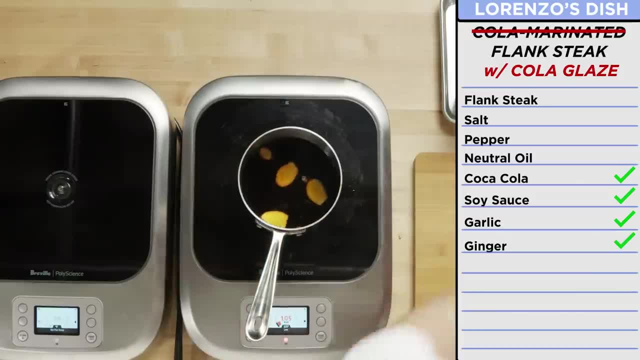 And I'm gonna look for this. Right now the bubbles are gonna be really small and kind of fluttery, And then, once this starts to get a little thicker, you're gonna see bigger bubbles that take a little longer to burst. You want to just reduce it until it starts to thicken. 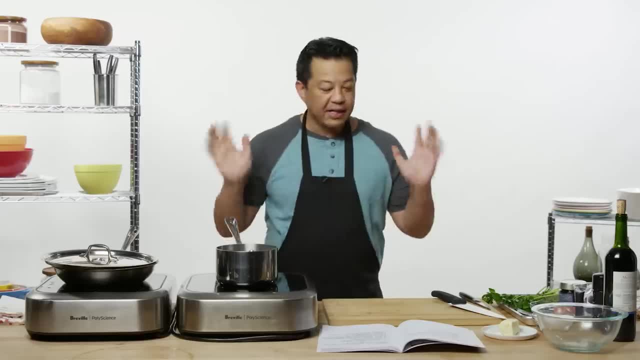 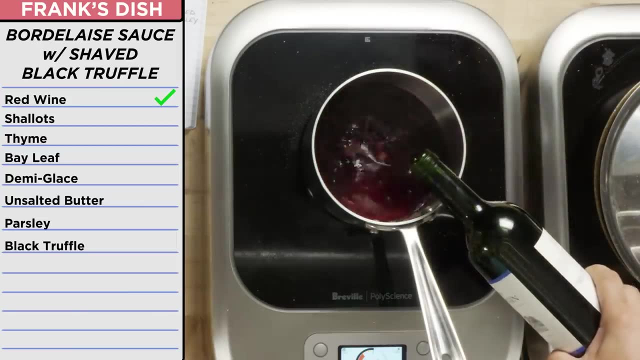 rather than until it's dry. If it gets dry it's gonna burn. All right, now I'm gonna do the red wine reduction, So I need to reduce this about a cup. Frank says It's about a cup, a little bit more than a cup. 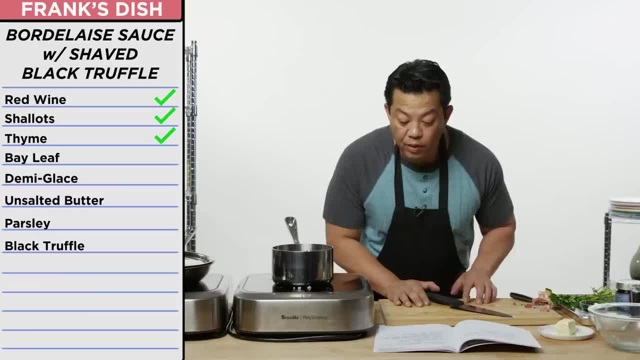 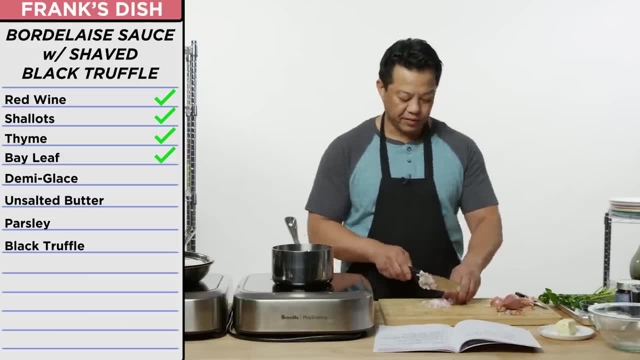 I'm going to add my shallots, fresh thyme and what-a-what-a-what-a-what-a-what-a bay leaf. Easy peasy. So far, so good. Ow, no, just kidding. Let's put a couple of these in. 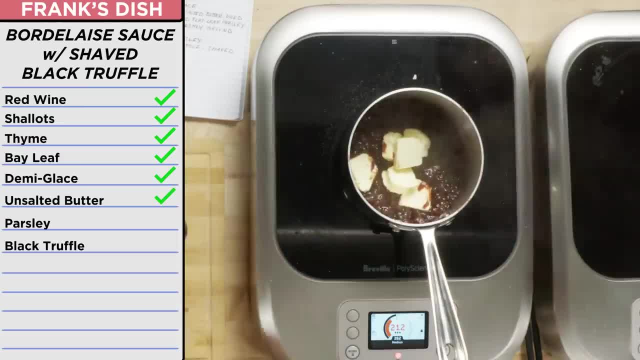 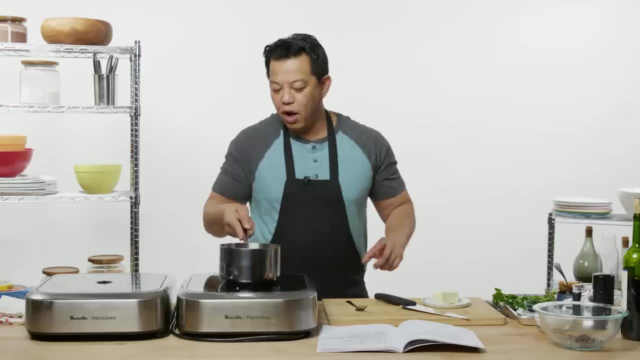 We can also. that looks like a very rich sauce. The color's fantastic. Not quite sure how thick it's supposed to be. Earth calling Rosemary. come in, Rosemary. What did she say? Can I ask you one more thing if you have time? 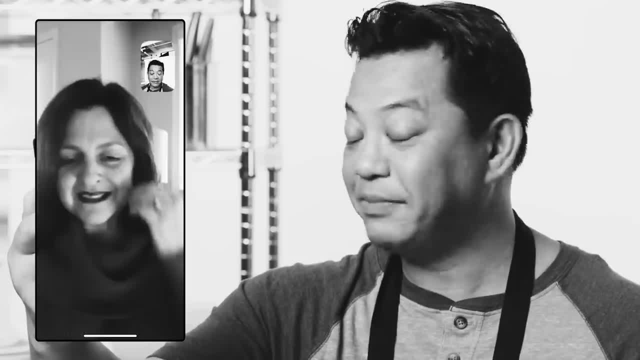 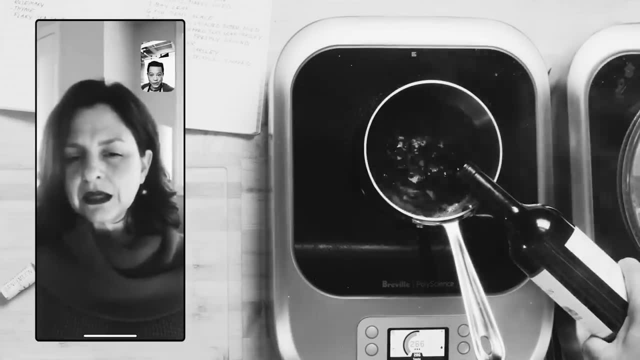 Okay, sauce. I have sauce that he wants me to make. I'm telling you what Frank is not getting: the Christmas card this year. I'm telling you, It calls for one cup of wine. How much do I reduce that? So stick a spoon in and then run your finger. 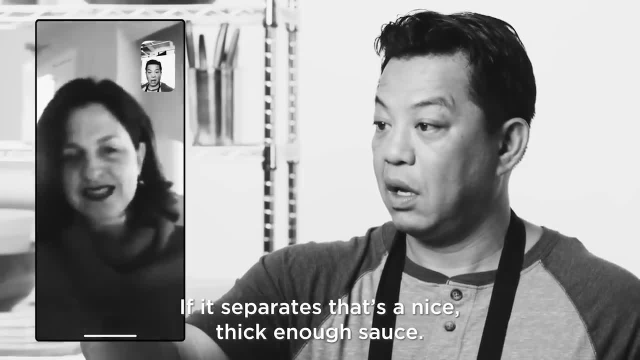 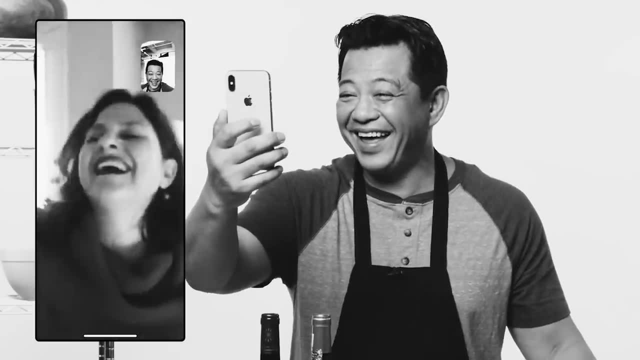 down the back and if it hates, that's a nice thick enough sauce. Okay, if not, worst case scenario, just drink the wine when I'm done. That is the test she wanted me to do, the old back of a spoon test. 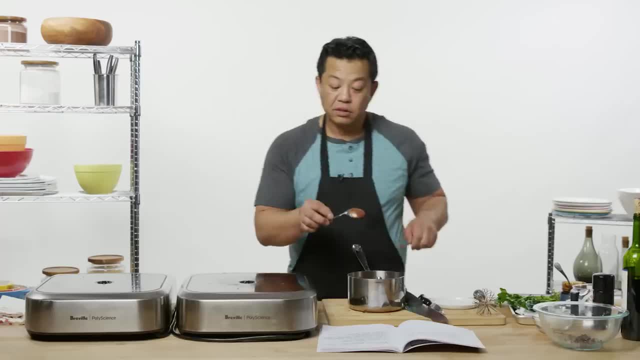 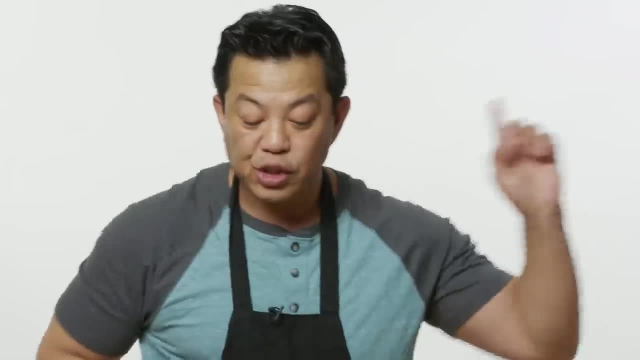 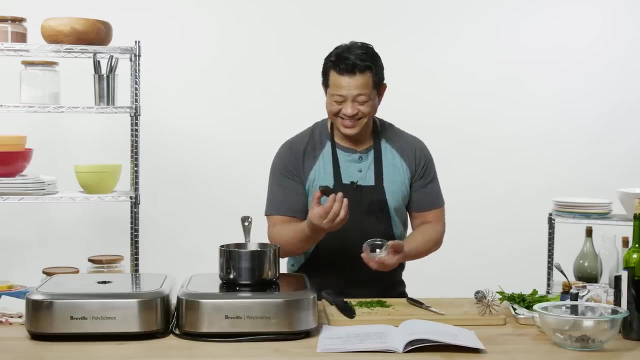 And if it leaves a nice clean line, I know my sauce is thick enough, Totally coated with a spoon. Thanks, Rosemary, Turn this off, and all I have to do now is shave some black truffle. Oh wow, never had one of these guys in my presence. 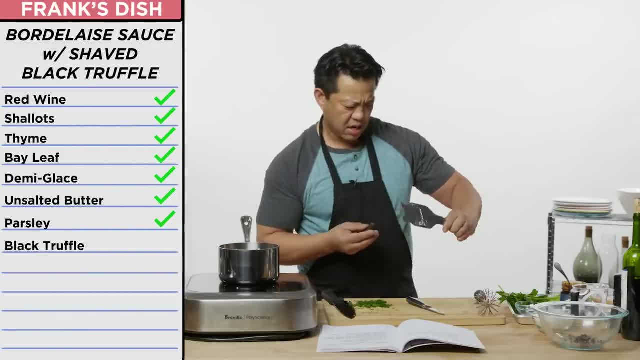 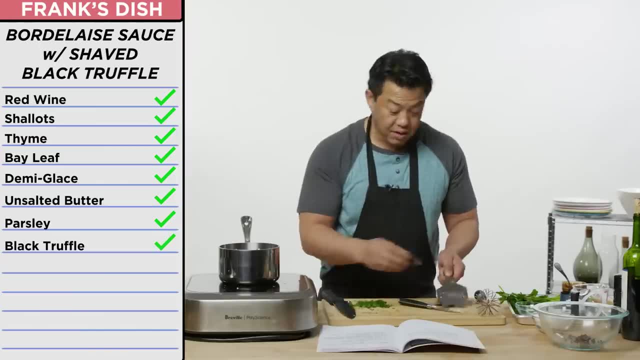 It's very it's earthy With truffles for the most part, they're best when they're freshly sliced on top of things. See, how much does he want us to do? Oh, the whole thing. Wow, There's truffle products that have. 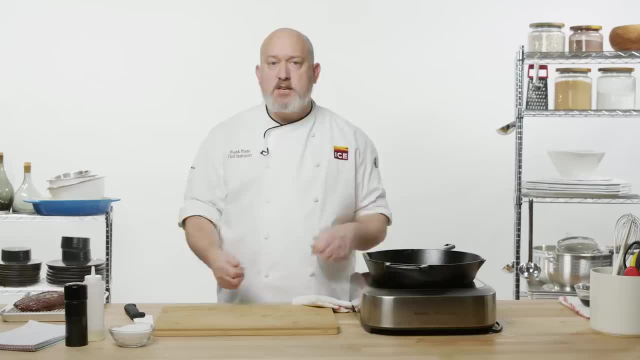 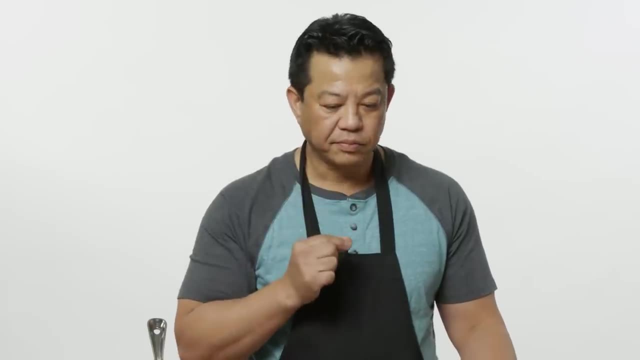 kind of those truffle flavorings in them. But when you get a fresh truffle it should be sliced at the table in front of your guests. It's not just for the flavor, it's for the show as well. It tastes expensive. 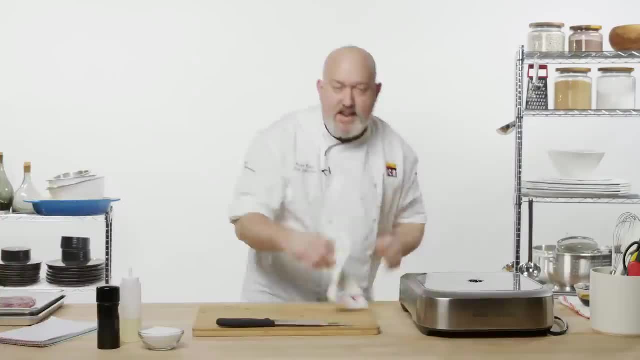 All right, guys. bordelaise sauce with black truffles. The next step is to do our steak. This steak is enormous. I mean, you guys Now, with the rib eye that I had planned, the high-end rib eye I had planned on sauteing it. 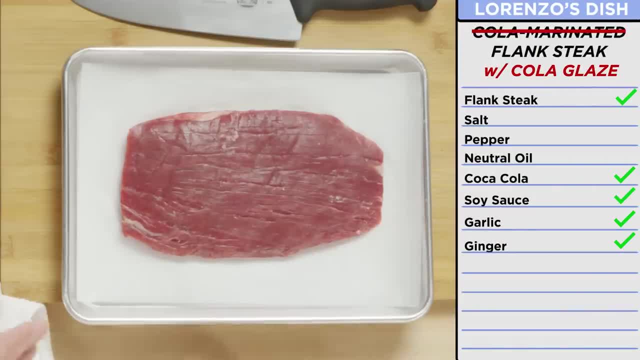 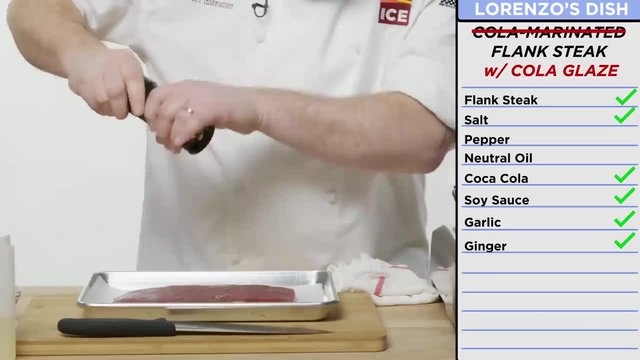 in a cast iron pan. The way I'm gonna cook this flank steak is similar to the rib eye. I really just wanna get a nice kind of caramelized coating on it, So I'm gonna season the steak first. A fair amount of salt and black pepper. 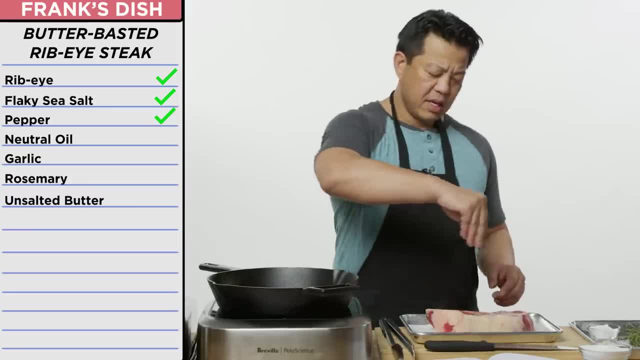 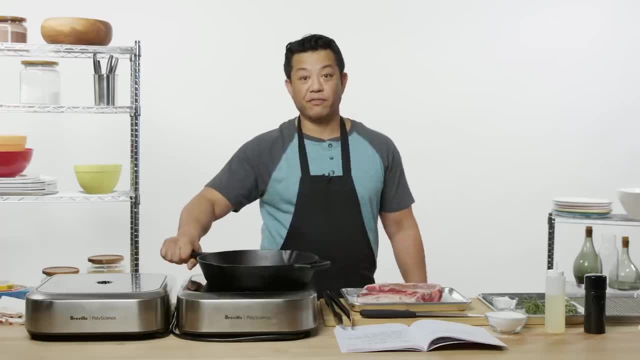 With the salt. we go fairly heavy Liberally, liberally, liberally. So I need this hot like super hot. you guys. This is the nicest skillet I've ever seen in my life. I like this. Christmas presents, please. 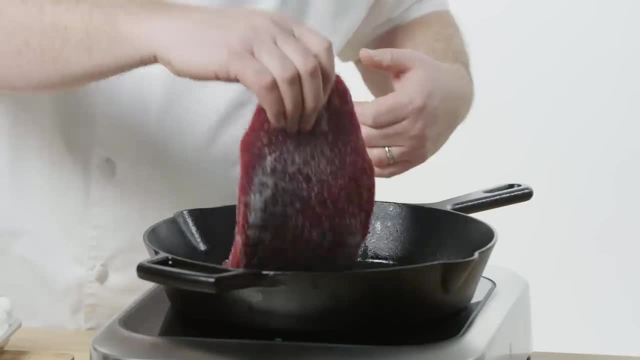 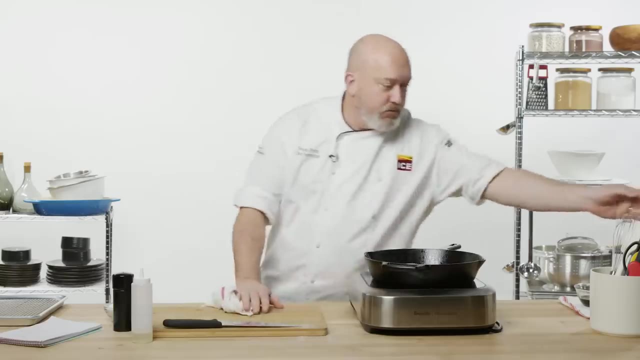 The key to this is that you don't want the oil to splash on you, so I'm just gonna drop it in the pan away from me. Here we go, guys, And I'm gonna let it stay there. Leave it alone, Let it go. 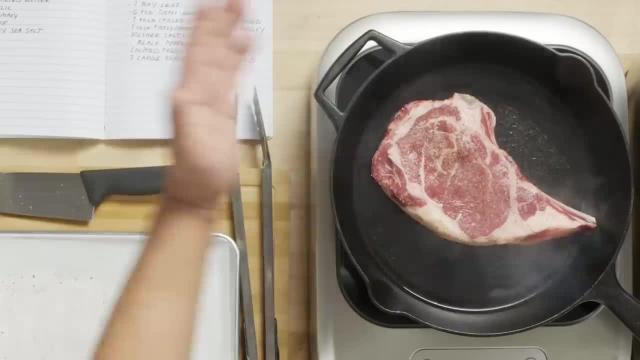 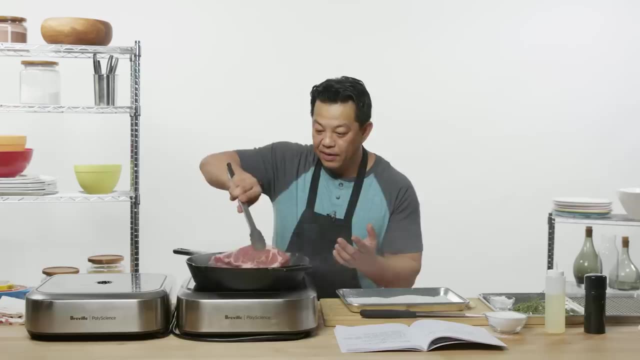 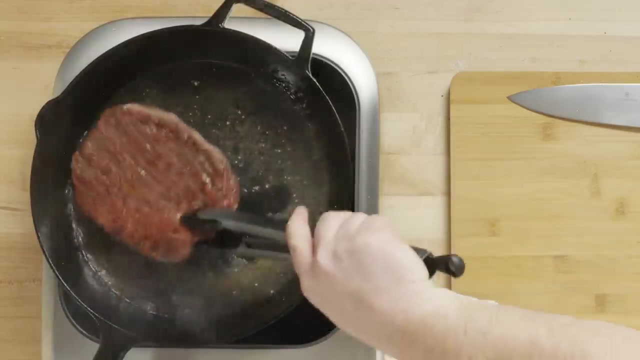 This is gonna take a few minutes. Send these smoke signals. Dinner's almost ready, people Come and get it. I'm gonna flip it away from me, Swirl it around so I have some nice amount of fat. If you look at the steak, it has a beautiful crust on it now. 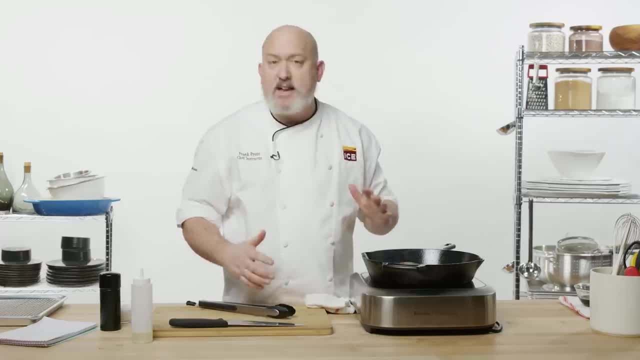 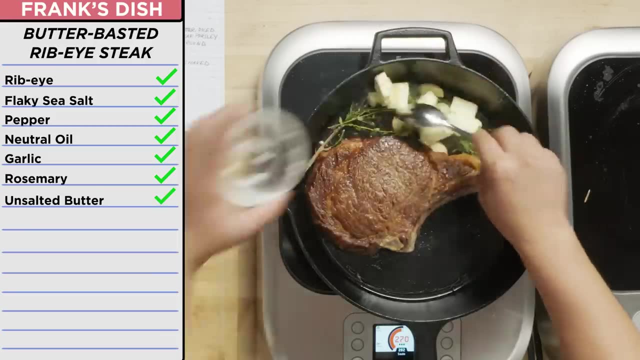 It's gonna add a ton of flavor to this steak. It's going to add some texture as well. You're gonna get a little crunchy bits. Let's just throw these in. We smashed it. What I'm gonna do to check temperature is I'm not necessarily gonna use a thermometer. 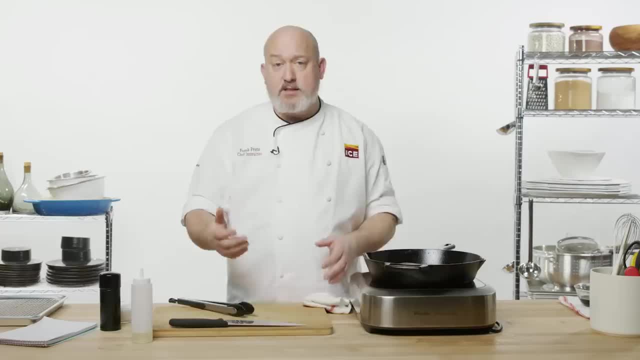 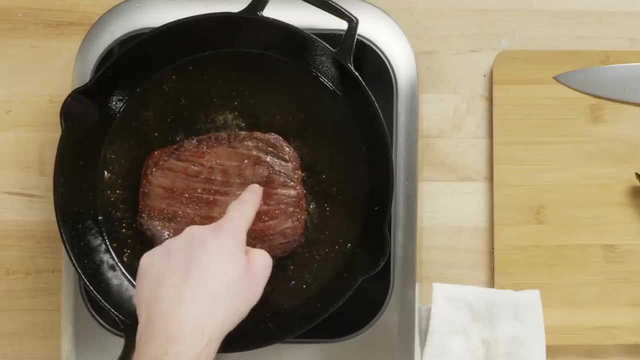 If I push on this piece of meat and it gives me some spring back, that means that it's cooking. If I push on this piece of meat and it leaves a dent, that means it's pretty much raw in the center. So this, I know, is still pretty rare here. 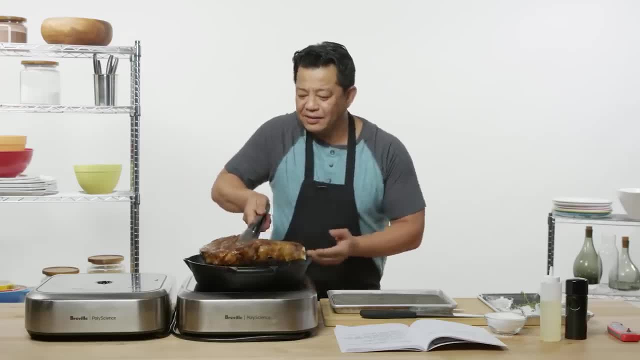 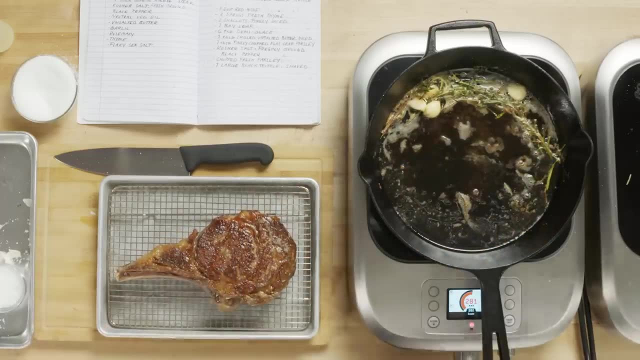 and here it's kind of cooking up: Guys, you guys, you guys, you guys. I think I'm teary-eyed a little bit. It's so beautiful, I'm crying. It's so pretty. Lorenzo's issue is gonna be. 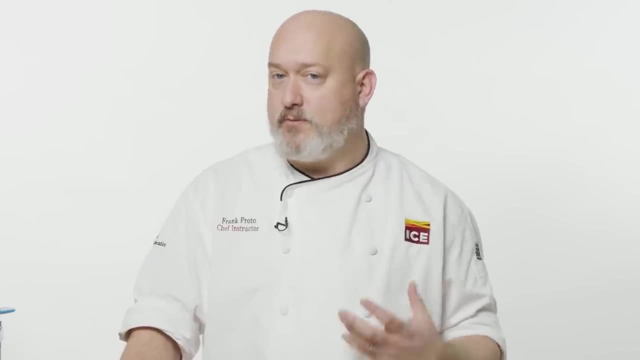 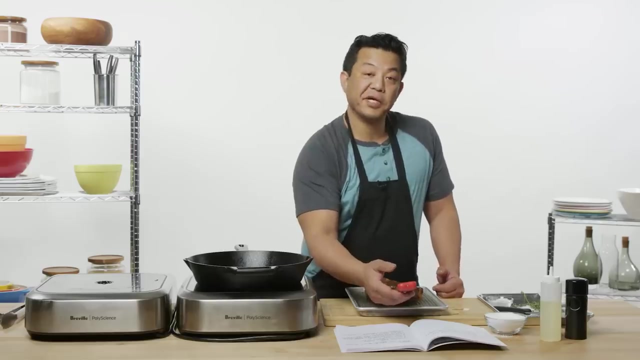 that's a really thick cut of steak And usually with those, getting the right temperature is a little more of guesswork. So Lorenzo might wanna use a thermometer for that. Ooh, medium rare, Perfect. So I'm gonna let this steak rest for about 10 minutes. 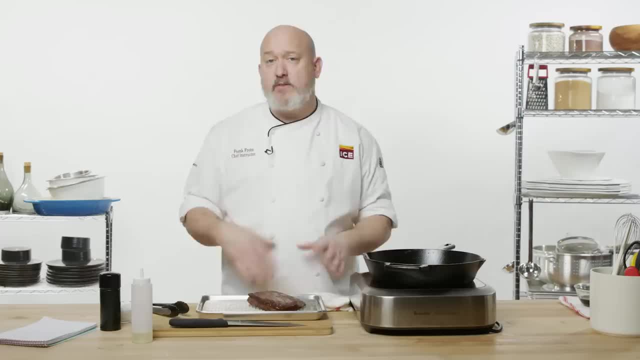 I really wanna dig in and eat this. I'm gonna eat this right now, but you need to let it rest. If I slice it now, all the juice is gonna flow out. Be patient, It'll be worth it. Let's move on to the broccolini. 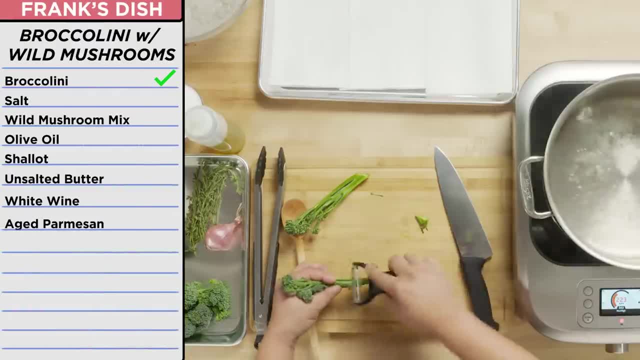 The expensive version. I was gonna use broccolini. We have a rich steak, a really rich potato dish, and the broccolini's gonna have just a little bit of bitterness to cut that. Broccolini tastes really great by itself. 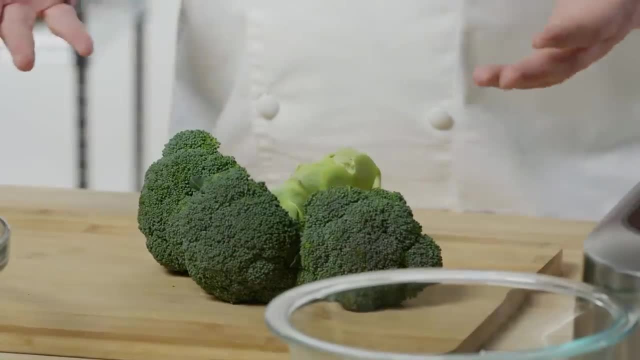 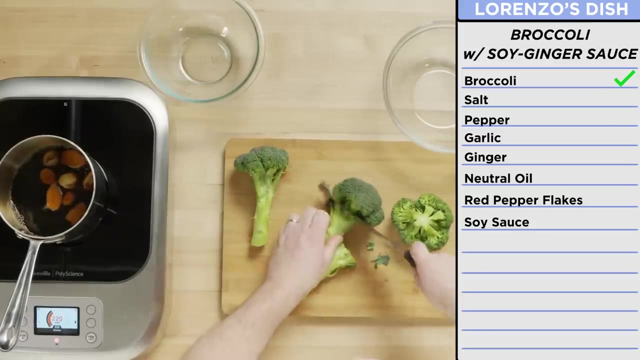 Needs a little salt pepper, maybe a little garlic. but everyday broccoli is delicious if you treat it right. So normally people take the broccoli, cut the head off and everything else gets thrown in the garbage. What I like to do is I save the snails. 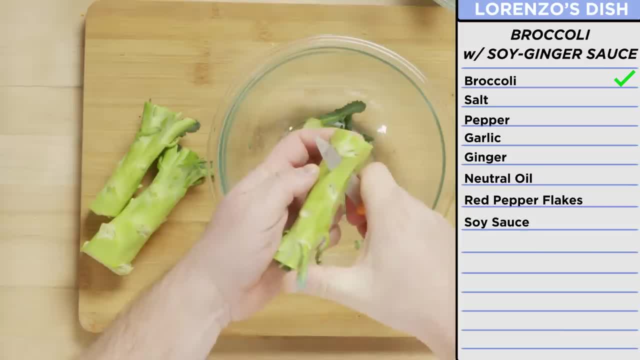 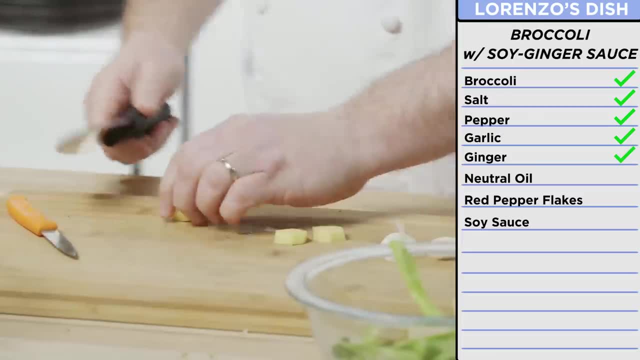 So if you're gonna serve the stems, you have to peel them, because otherwise it's a little on the tough side and it sometimes needs a little help. So what I'm gonna do is I'm gonna get some garlic and a little bit of ginger. 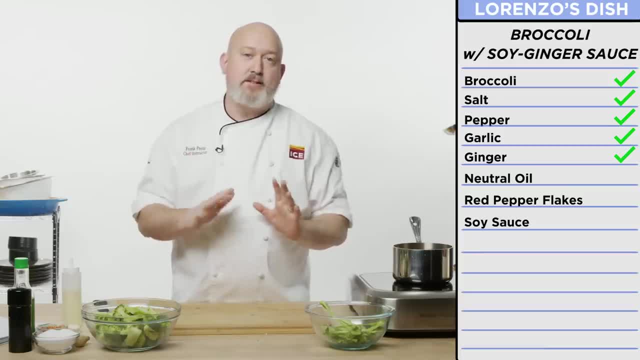 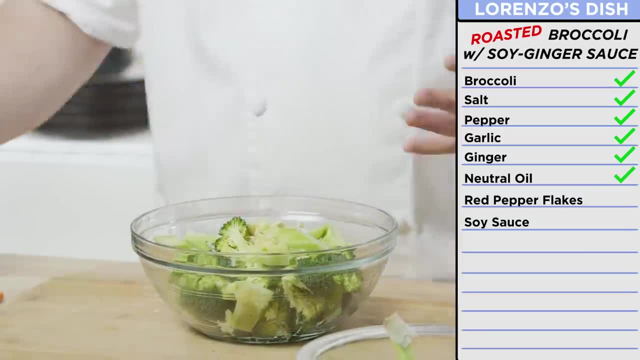 A lot of times people will boil broccoli and boiled broccoli. I mean. there's nothing worse than that, right, It smells bad, it tastes bad, it gets too soft. I like to roast broccoli. It adds a little bit more depth of flavor to it. 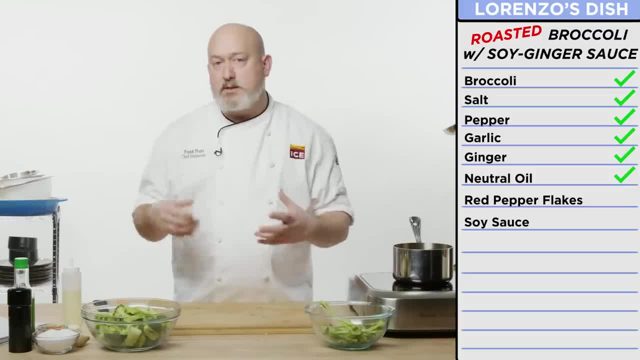 and I'm gonna use some of Lorenzo's ingredients here to make that just a little bit better: A little bit of chili flakes, just to let them know it was there. I'm gonna use a little bit of soy sauce, I'm gonna use a little bit of salt. 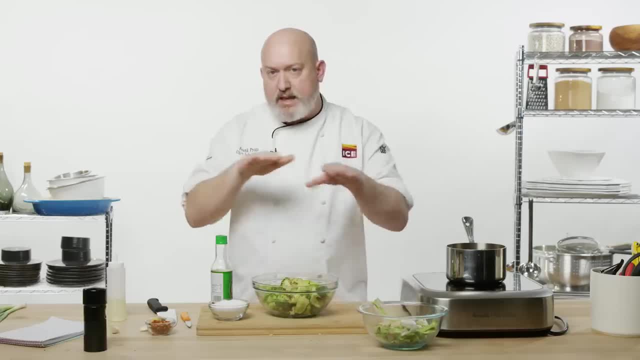 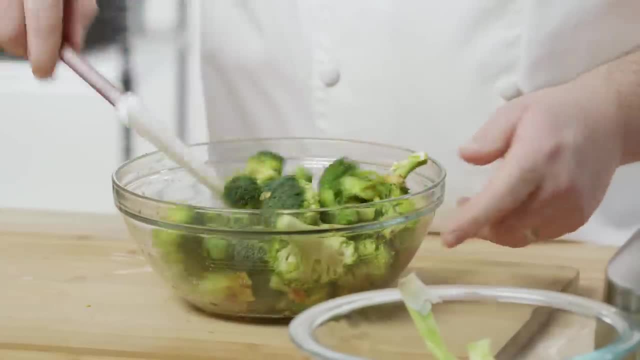 Both of them have salt in them, but salt kinda gives a pure, plain flavor, where soy sauce kinda gives a richness. I'm gonna throw this into an oven- about 350, for about 15 minutes You'll see the broccoli starts to break down. 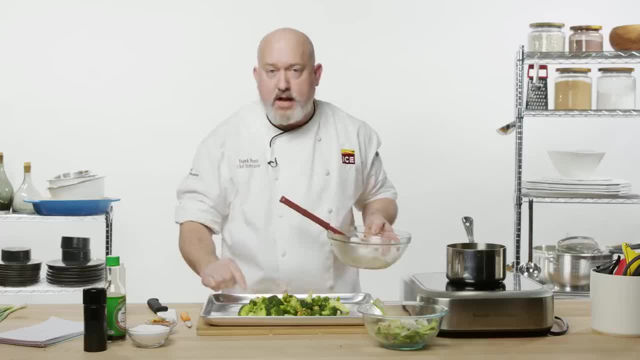 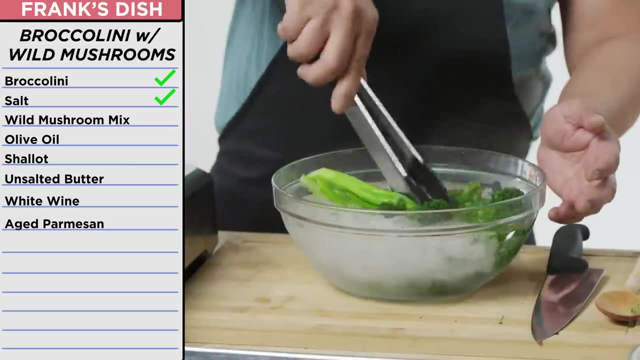 It'll start to get a little bit of caramelization or charring on top, and that's what I want. I wanna take it out of the oven when it's just a little bit crispy. I'm actually going to take it out, stopping the cooking process by submerging it into ice water. 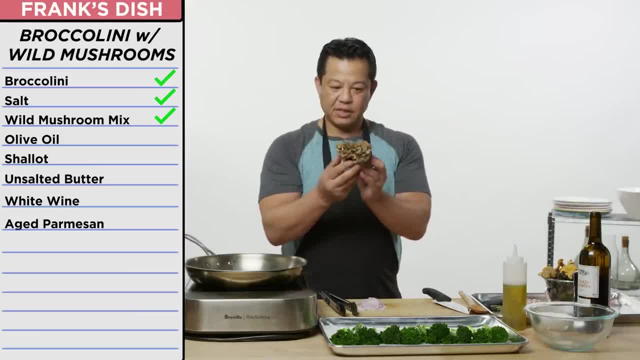 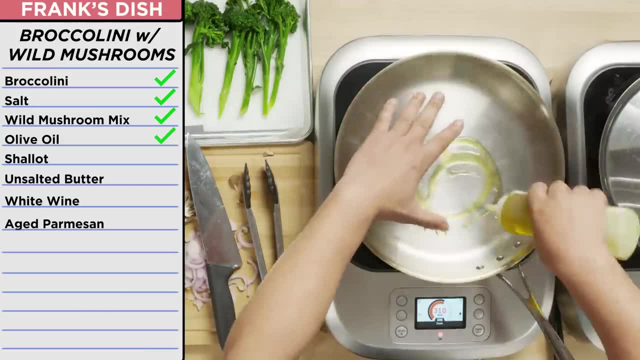 I think that's gonna be the best Mushrooms. I just have to start seeing what these are. These are great. Lorenzo should make sure that he gets those mushrooms nice and caramelized. Any mushrooms that kinda go in a pan and they just kinda sit there and boil, not good. 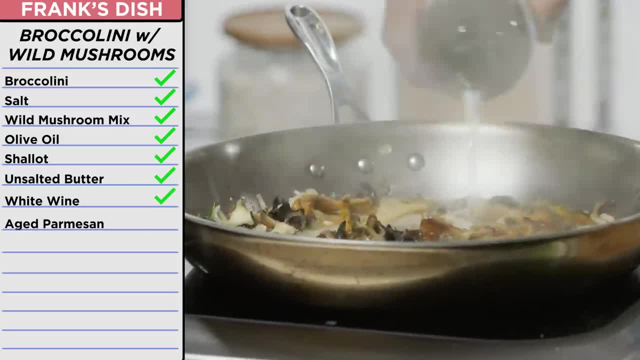 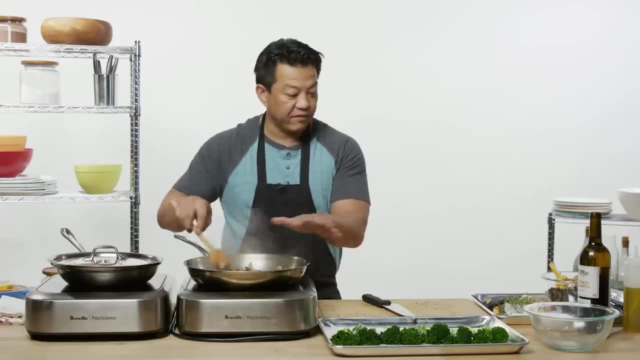 The texture's not really great. You want those mushrooms to be just slightly crispy when you put them on the plate. These are very thin, delicate mushrooms, so I think it's okay to add whatever I need to add to finish this off. My broccolini looks good to me. 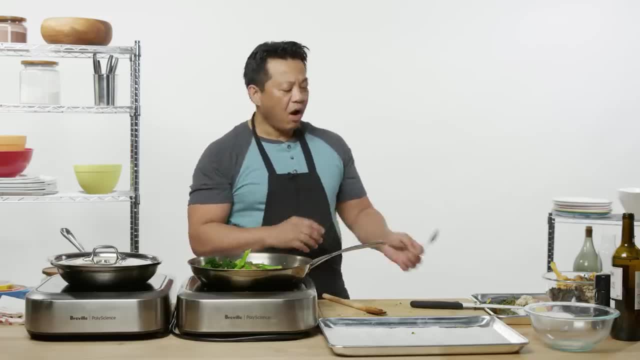 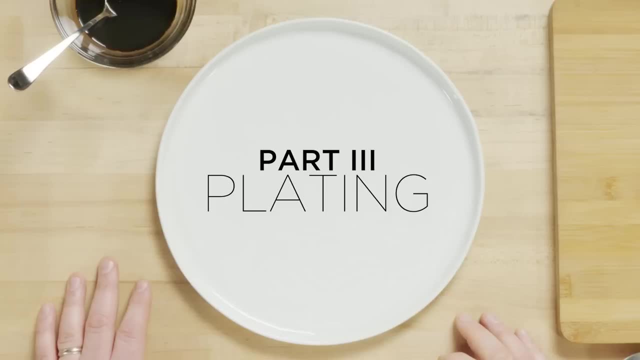 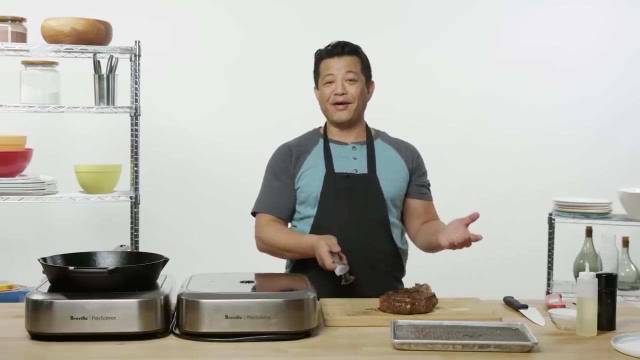 Let's try it. Wow, This is lovely, Lovely, lovely. jubbly is all I have to say. And wow, it's heavy. It hurt my wrist it's so heavy. The most important thing for this piece of steak. 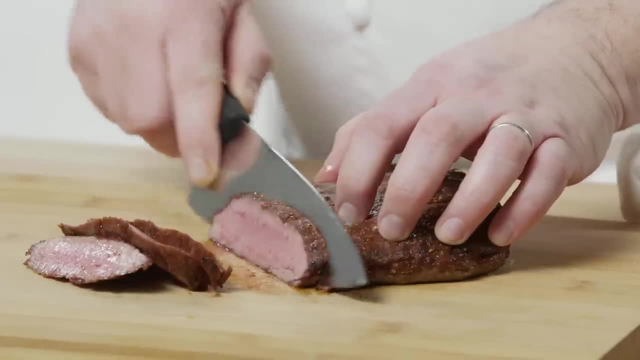 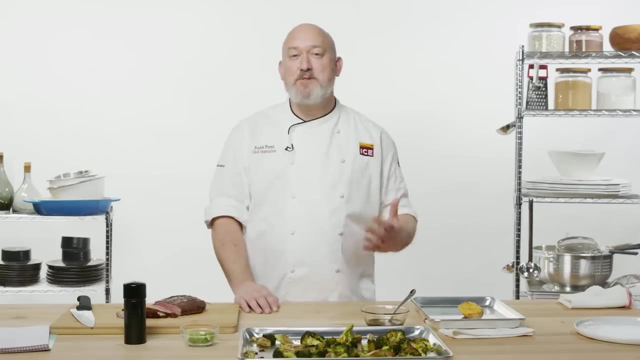 is to cut against the grain. That's because if you cut it with the grain it's just gonna be super chewy. It looks so good. Does it look good? When I'm plating a dish, I'm usually looking for a little textural difference. 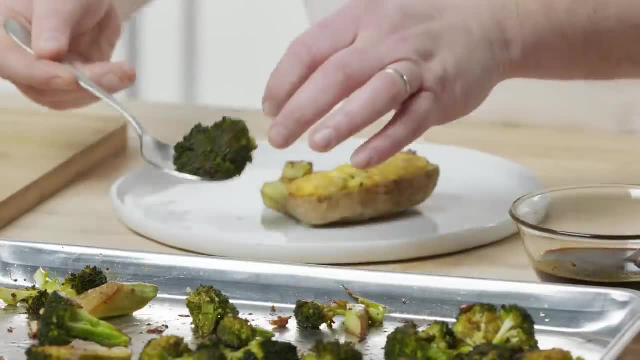 a little height difference just to make it interesting. If you just throw everything on a plate flat, it's kinda boring. So I'm gonna kinda just prop things up a little, do a little chef wizardry and try and make it. 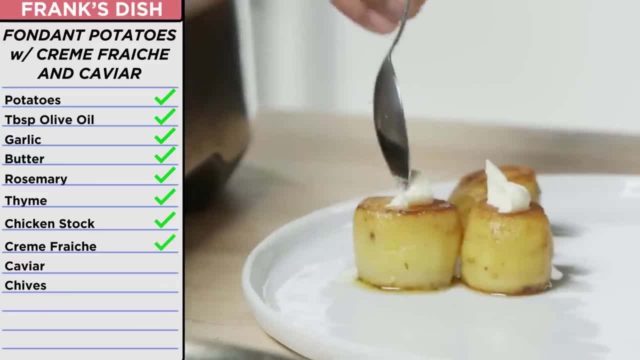 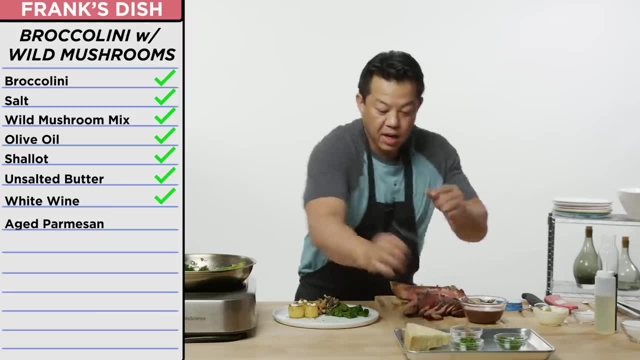 just look a little bit nicer than what kinda grandma would've put on the plate Fresh caviar. Ooh, it's the green caviar. Let's put a little bit of chives on this, guys. Oh, Broccolini has shaved fresh Parmesan. 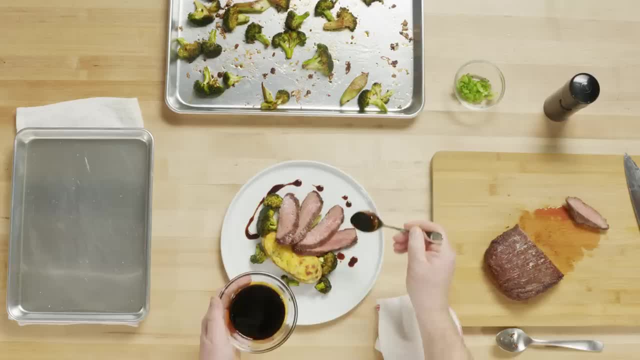 So we have our beautiful steak propped up on our broccoli stems. I got a little bit of that soy and Coca-Cola glaze and that's my take on Mr Lorenzo's dish. There's a little piece left on my board. 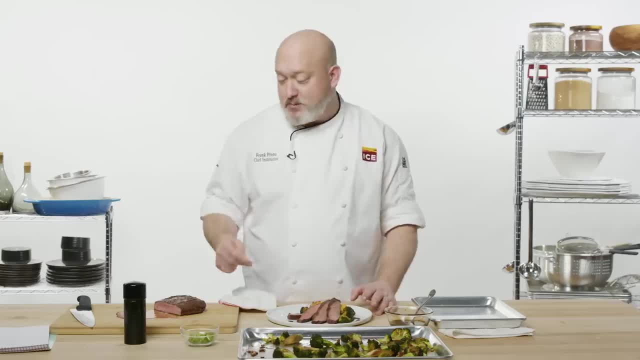 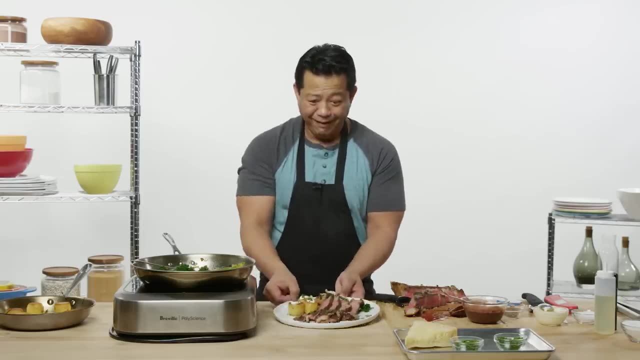 That's the chef's secret. We eat all the ends. We make staff meal out of it sometimes, but that's my snack. okay, Truffles and uh, That's it. That looks good, man, If I do say so myself. 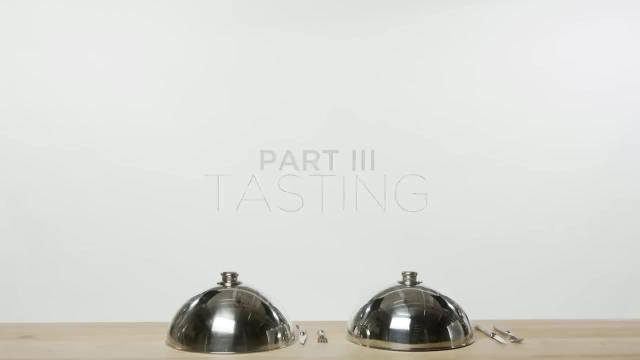 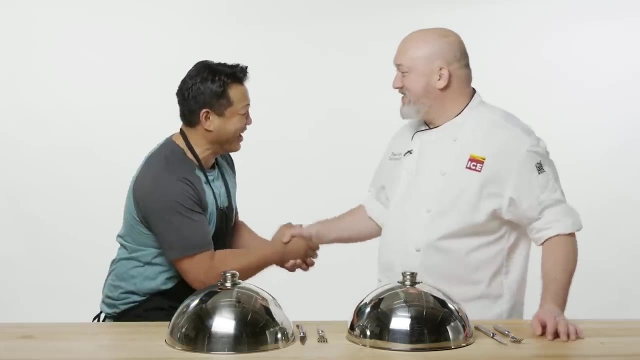 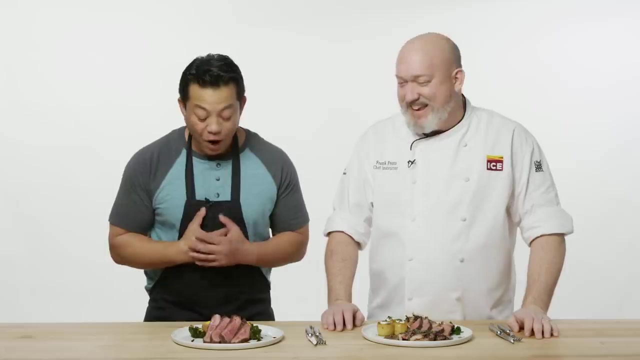 Steak. Hey, how you doing, Frank, it is an honor and a pleasure, Pleasure to meet you. I'm telling you right now, sir, Pleasure to meet you. Well, look at that, It looks good. Oh, that is my potato. 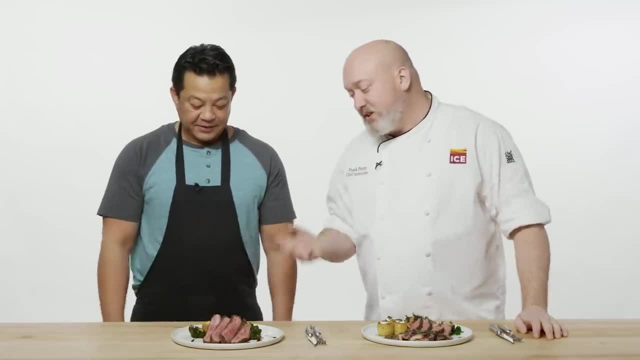 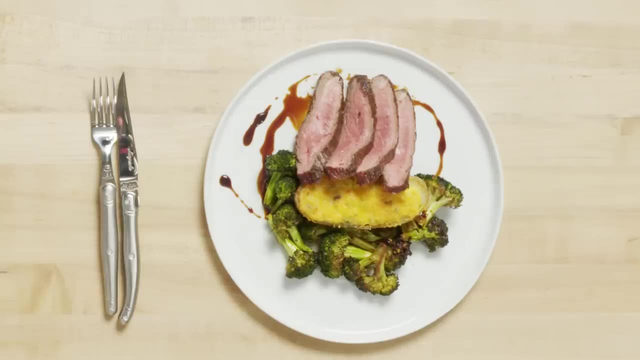 Oh, it's a twice. Yeah, So you know, we took a little chef's poetic license with this right. Yes, you, We made like a little glaze with the Coca and the soy sauce. Oh, very good, very good. 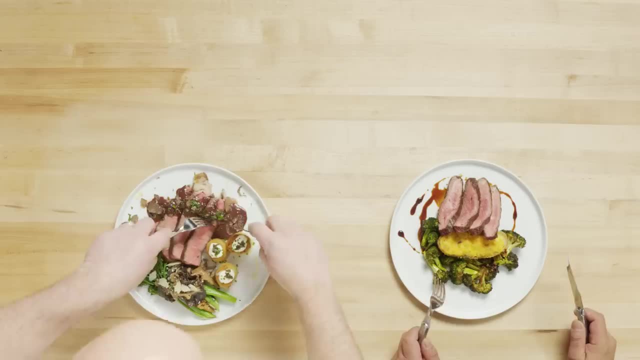 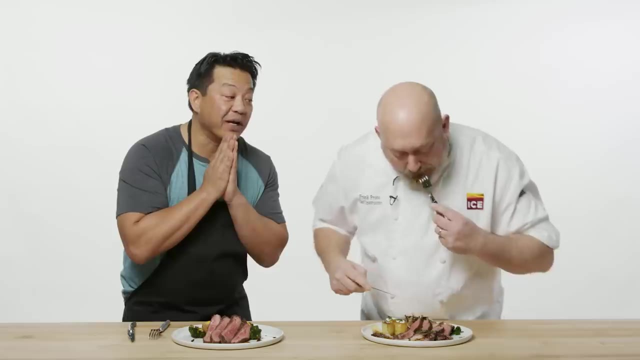 The broccoli we roasted with some ginger and soy And then we did a twice baked potato. So I'm gonna give it a taste with this sauce and a little bit of mushroom on there. Okay, I don't even know what kind of mushroom that is. 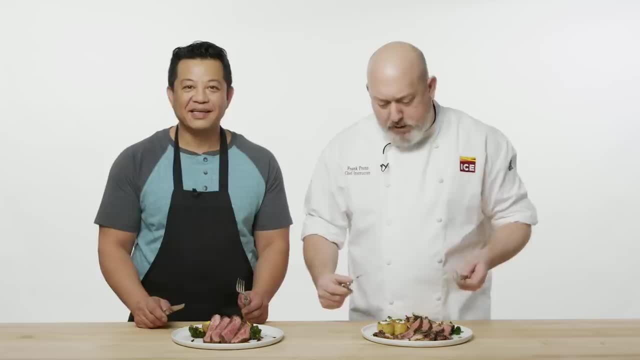 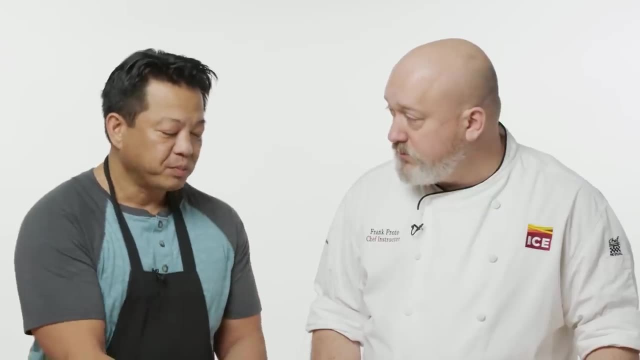 I think it's a chanterelle Delicious. Your seasoning is wonderful. Oh, thank you. Oh man, great, Really. Sauce is on point. I never had a sauce like this before. It's one of those classic French sauces. 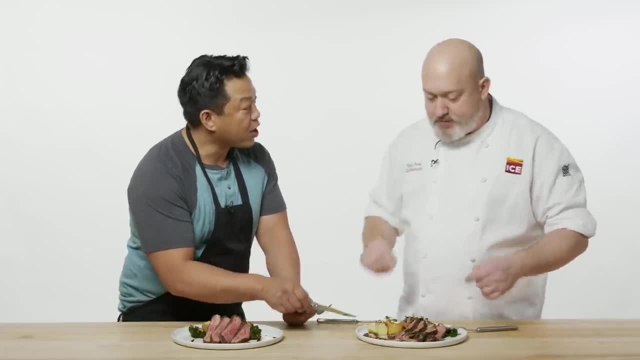 You know you would think it'd be too rich, but it actually is a good foil for the steak. It looks like it would be so, so rich. Because the color- look at the color. It's a great compliment. It's different. 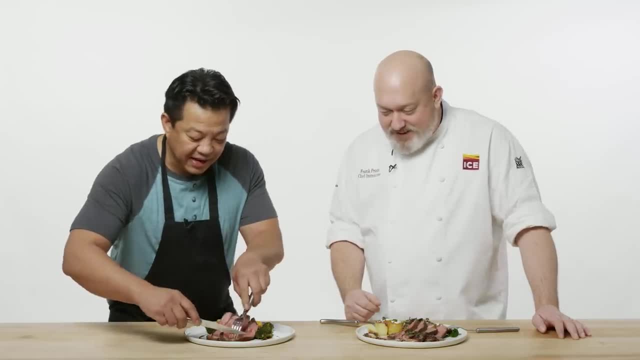 That is good. Let's taste yours now. Okay, Let us get a little bit of this. and your? I'm nervous too now. My heart's beating, I'm a little worried. What is the reduction? Is this like the soy sauce?